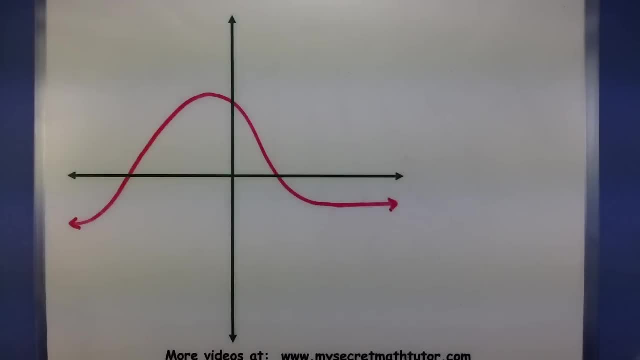 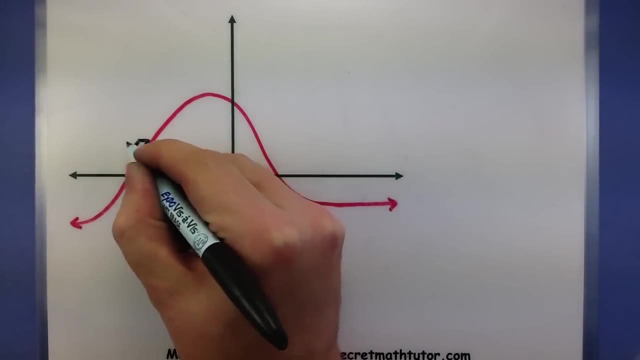 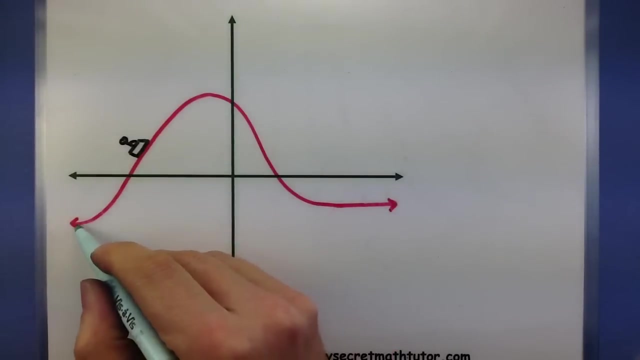 look at a function and see To get a sense of where this function is increasing or decreasing. I like to imagine that my function is instead a roller coaster And so when I'm looking at places where it is increasing, then I'm looking at places where I'm going up on my roller coaster, So I can see on this. 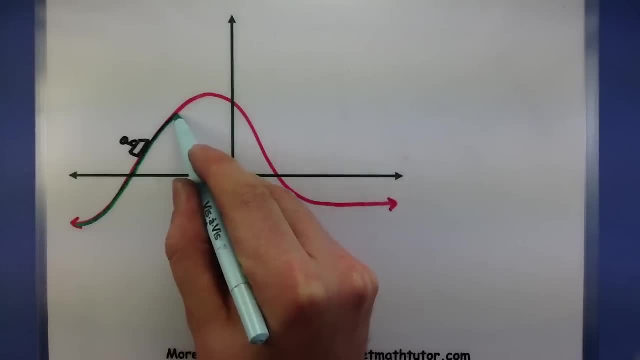 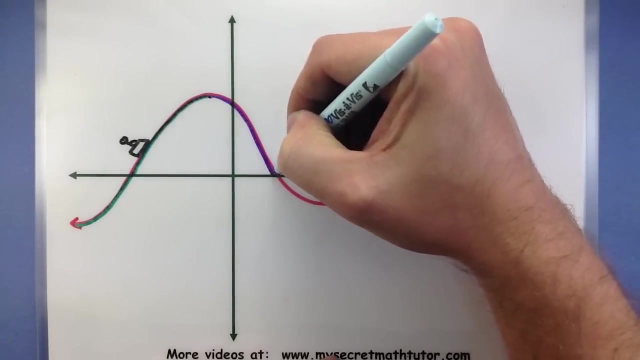 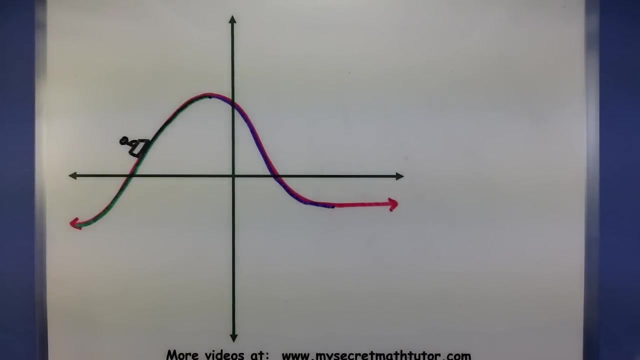 section. for sure I'm going up in my roller coaster Now. places where I'm going down those would be decreasing. So on this little portion of the graph I'm definitely going down And if it looks like my coaster is not changing, 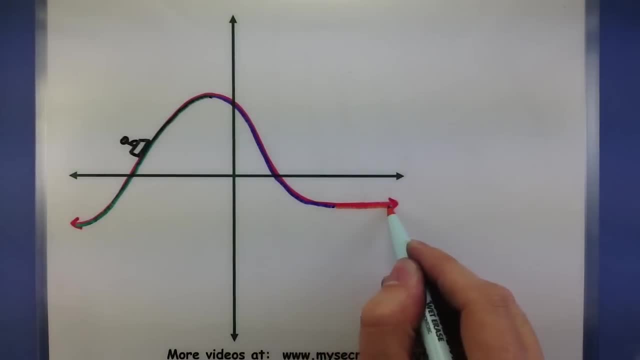 at all. I could say that it is constant. So maybe that little flat part over there is where the function is constant. Now, when it comes to describing increasing or decreasing, I like to think of it as a constant. I like to think of it as a constant Now, when it comes to describing increasing. 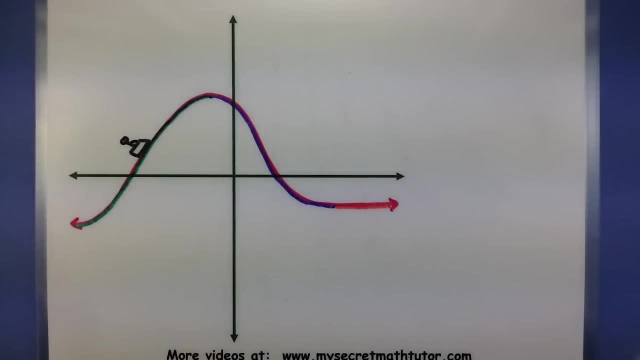 or decreasing. I like to think of it as a constant. I like to think of it as a constant. So when it comes to describing where these places are, we take things back all the way to the x-axis. So this point, where it changes, is my interval for increasing, because, on 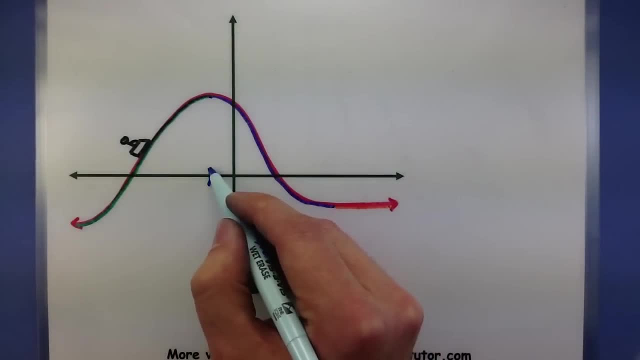 this entire interval I'm going up. After my little mark it looks like I start to go down and then eventually it goes constant. So I want to describe all of these x intervals as constant. So this is my interval for decreasing and increasing. This is the xx that I'm going. 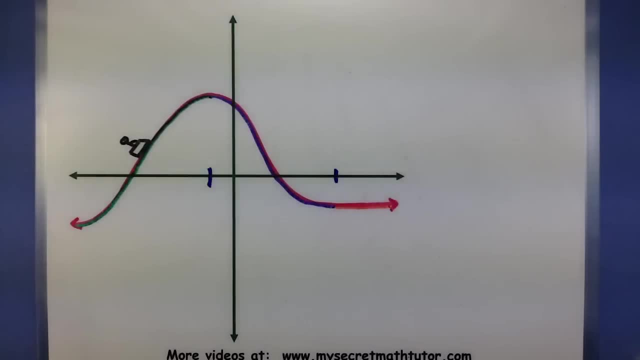 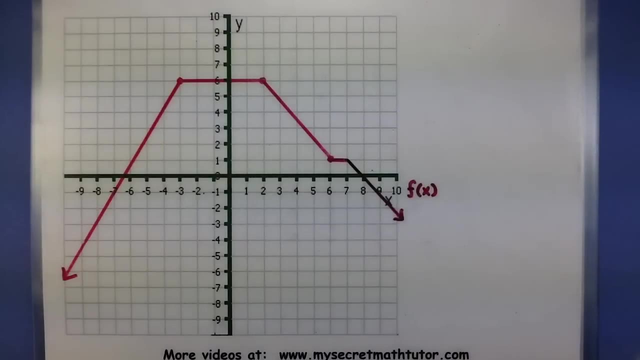 up to Now to describe increasing or decreasing. I like to think of it as an interval for increasing or decreasing. Let's get some more examples and be a little more precise with this. So suppose I'm looking at this function and I have to write down the intervals of increasing. 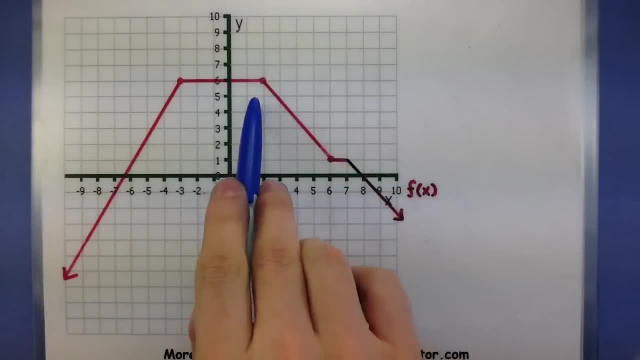 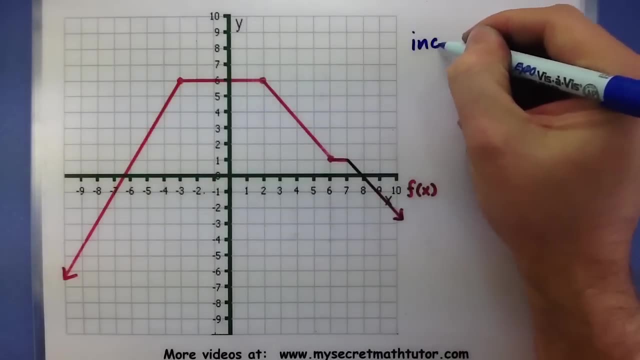 or decreasing. So think of the places you're going up on that roller coaster versus the places you're going down. Let's first track down all the places where we are going up. This is for increasing. Well, I can see this first portion. I'm definitely going up and that happens all the way until. 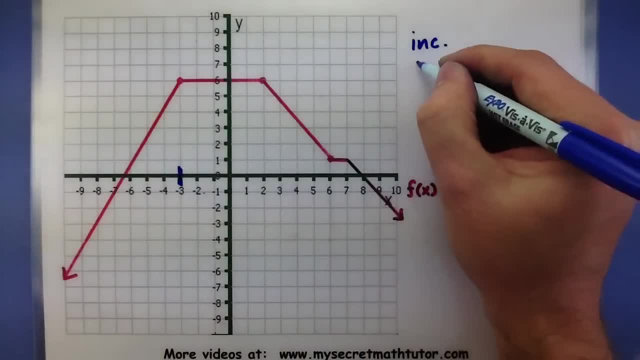 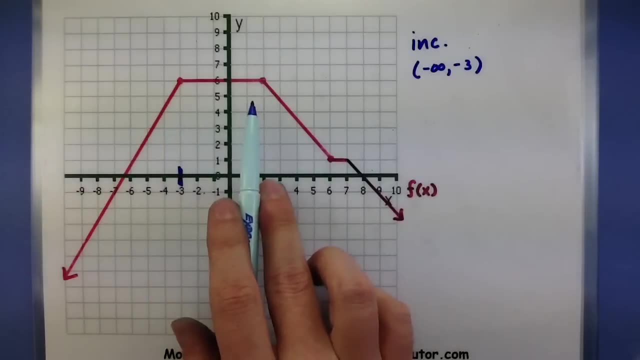 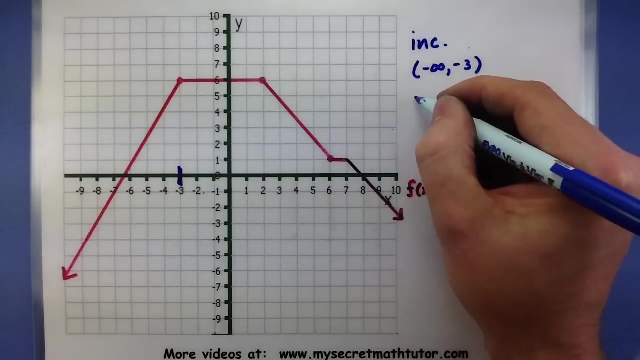 I hit a negative 3.. So using these x values, I can say that it is increasing from negative infinity up to negative 3.. Looks like it goes constant, down, constant and then down. So that's my only increasing interval. 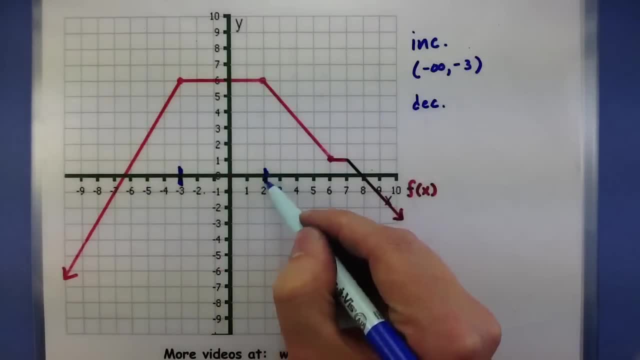 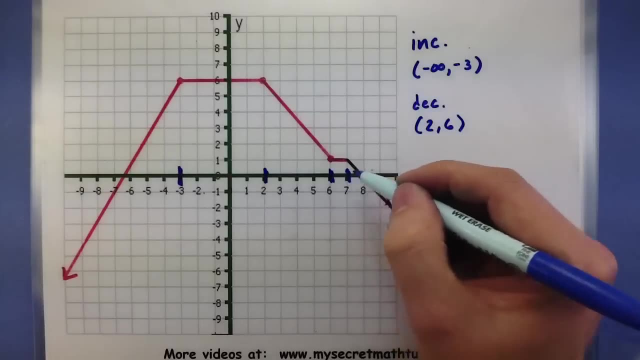 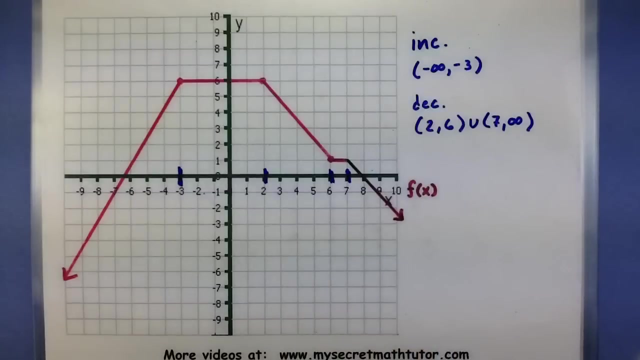 For decreasing, I can see that happens between 2 and 6, and it happens again from 7 onto infinity. So I have 2 decreasing intervals And of course we can also add places where we are staying constant, where we're not going. 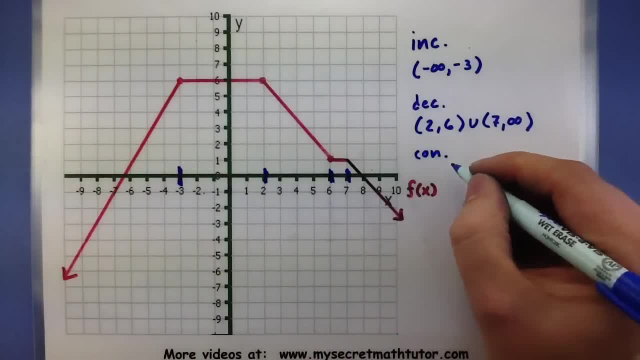 up or down and it's just our left-over pieces here. So from negative 3.. 0.. to 2, and from 6 until 7.. So 1, think of the places where you're going up or going down on that roller coaster. so 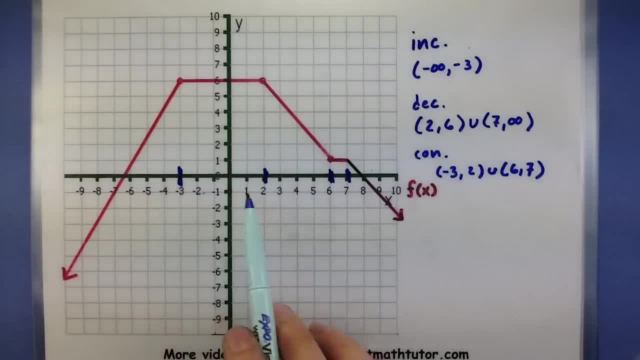 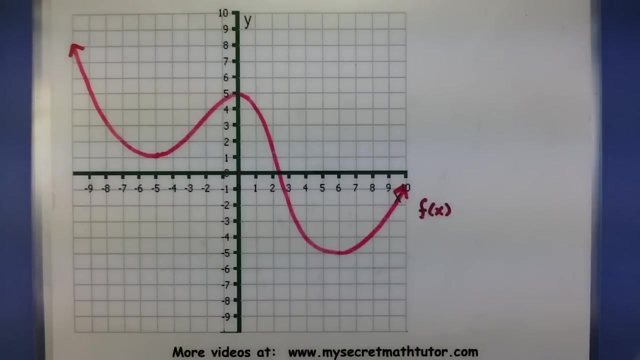 you just know your intervals. Take things back to the x-axis and describe them from the starting and end point. Let's do one more of these things. This one's a bit more curvy, but we can still go through the same process. 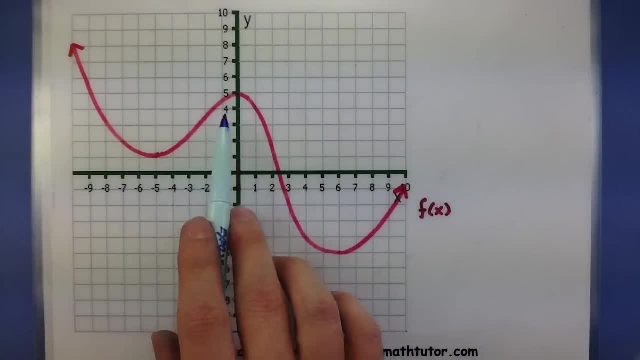 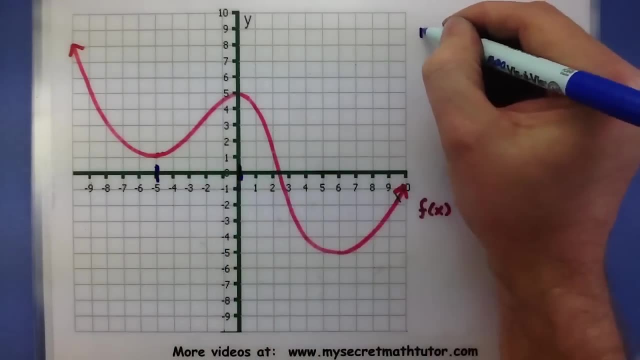 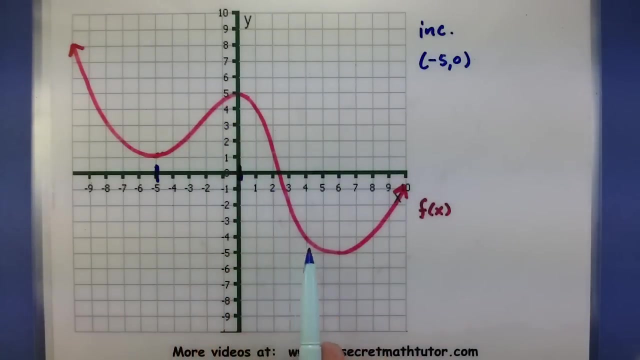 So first imagine where we are going up on this roller coaster. Looks like I have a little section here going from negative 5 all the way to 0. So increasing negative 5, up to 0. And my roller coaster goes down, starts to go up again after 6.. 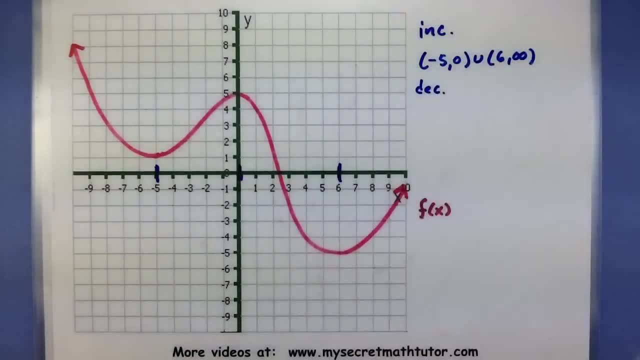 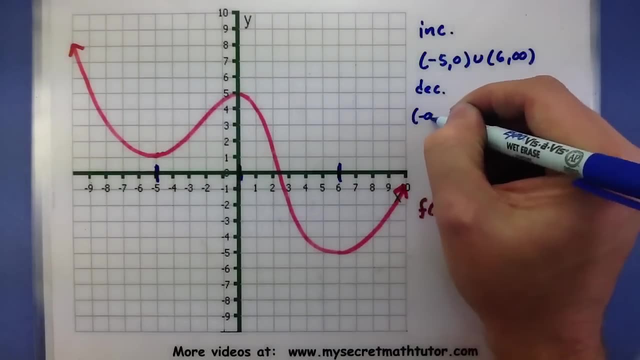 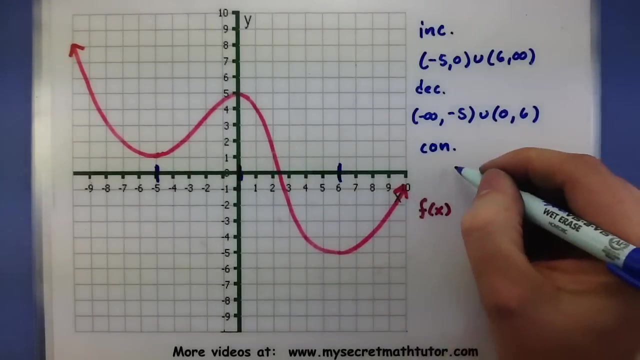 So two intervals for increasing On to decreasing. Okay, It goes: decreasing here, decreasing here, Negative infinity up to negative 5. And from 0 to 6.. As for places, that this place stays constant, I'm going to say none. 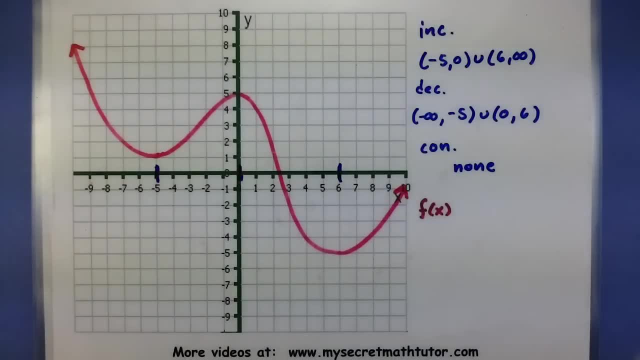 So hopefully that helps you out figure out where a function is increasing and decreasing, And this is an important thing. It's an important topic which you will definitely need for calculus.